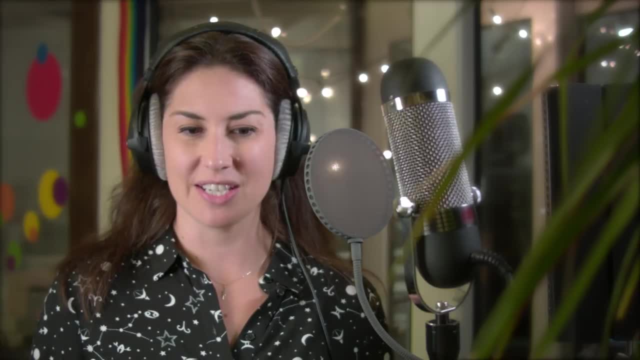 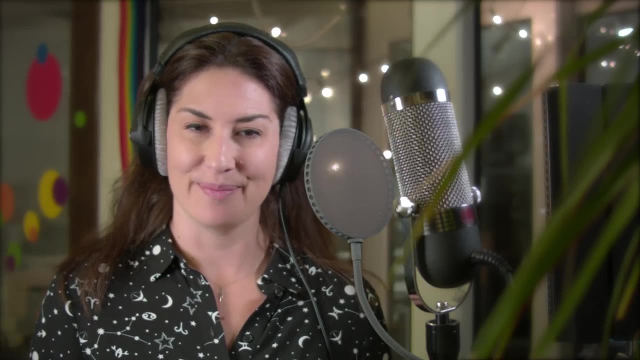 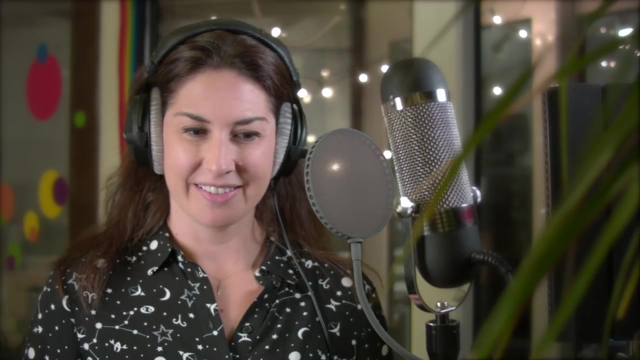 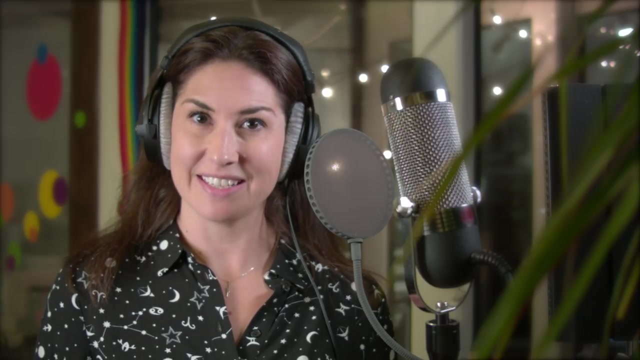 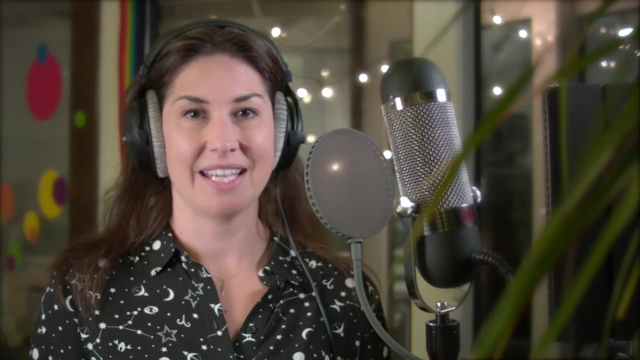 Take a little time for any last-minute wriggles or fidgets and when you're settled, let your body become still and calm There. Well done, Start to see if you can just notice your breathing. Can you feel it Rising and falling as it comes in and out? 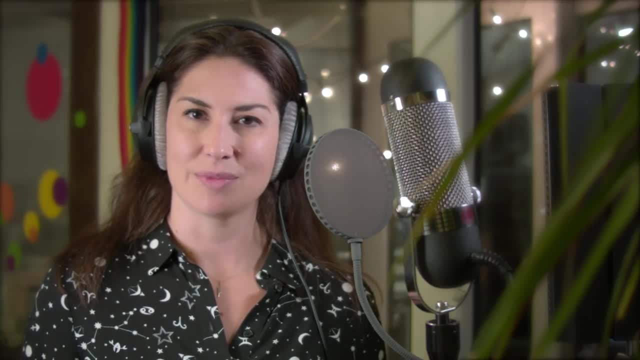 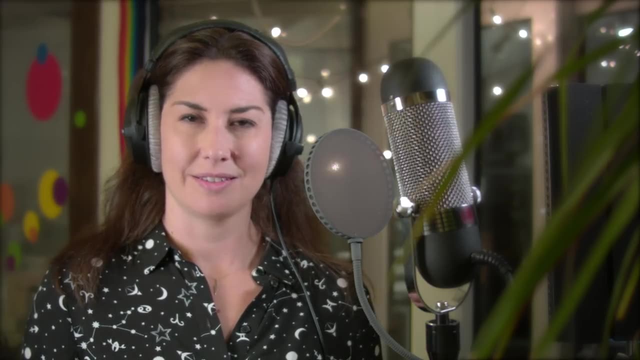 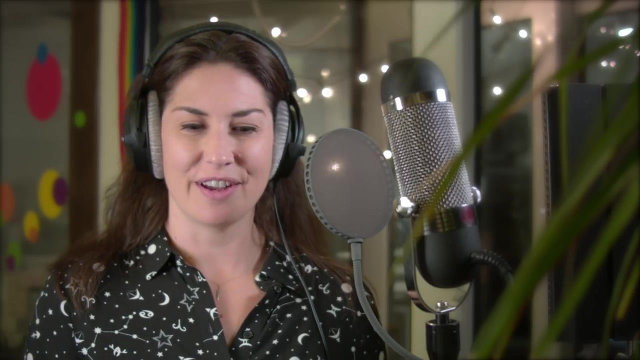 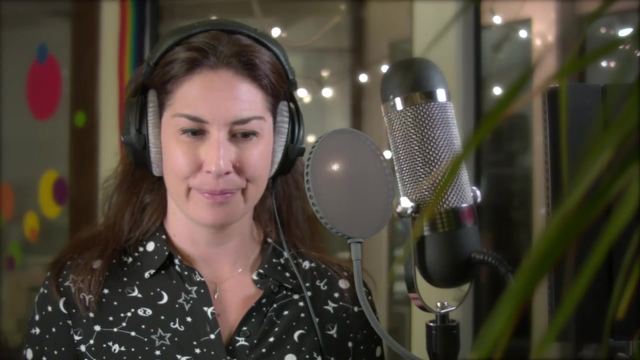 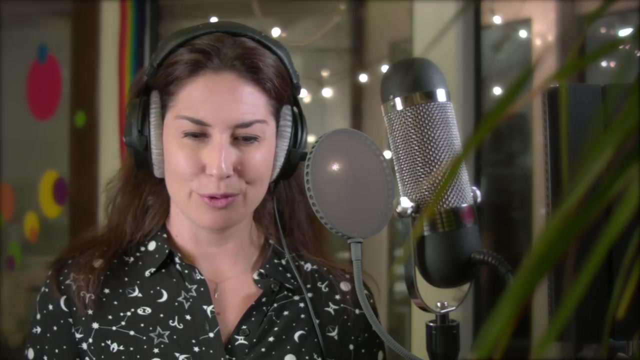 Just see if you can follow it as it comes in and goes out. You don't need to try. Breathing was the very first thing you learned to do as a baby, so it comes very natural to you. As you breathe and pay attention to it, you make your body feel all soft and relaxed inside. 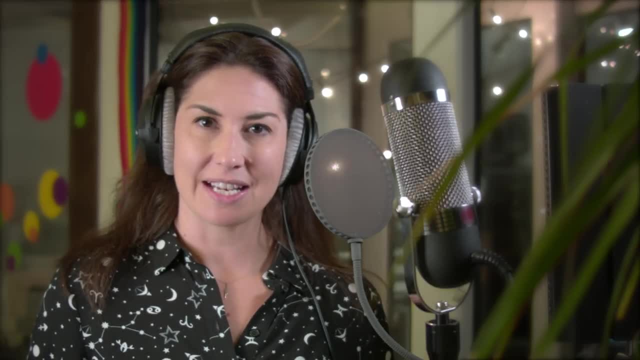 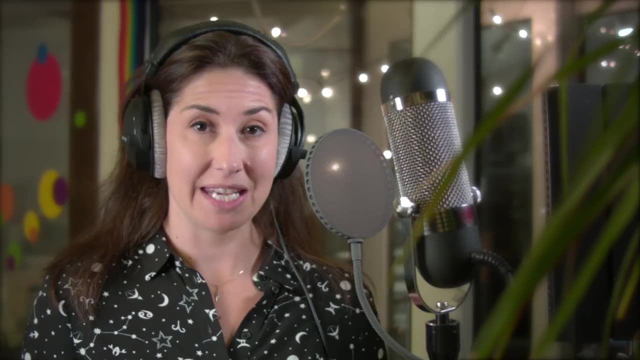 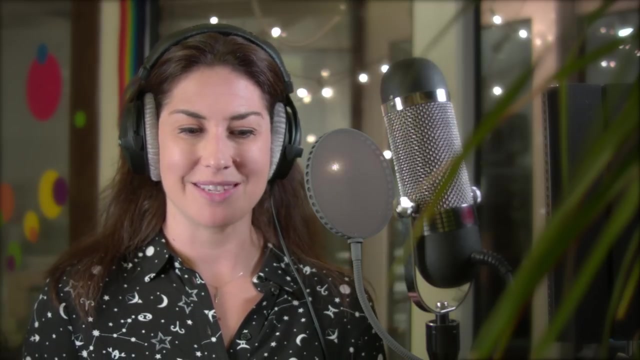 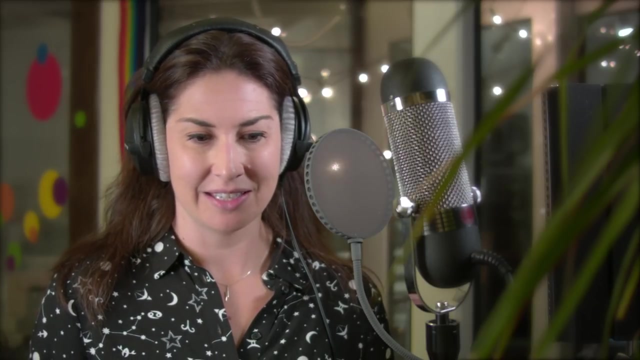 If you haven't already, you can gently, softly close your eyes. That often makes it a bit easier to notice our breathing. Now we're feeling all peaceful and relaxed. Let's enjoy going on a special journey in our mind. All you have to do is be here. 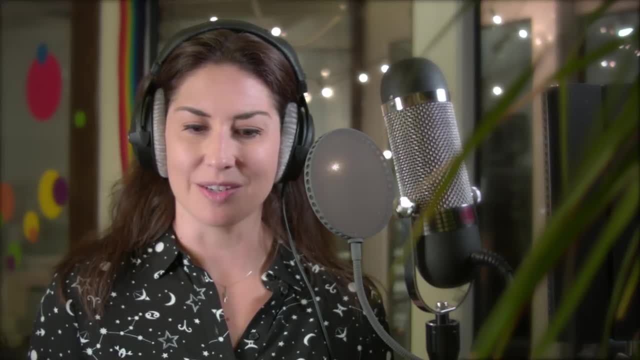 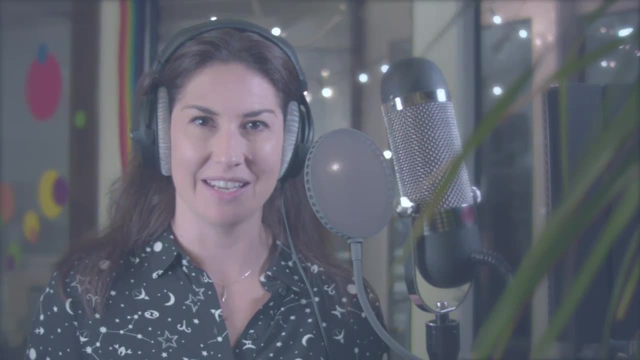 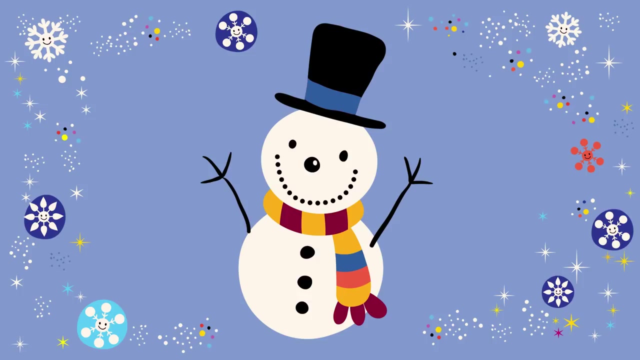 Listen And see if your imagination is working, And see if your imagination can make the pictures for you Like you're in a dream. Let's begin. It's winter And outside the snow is falling. You are inside, all warm and cosy, watching it through the window. 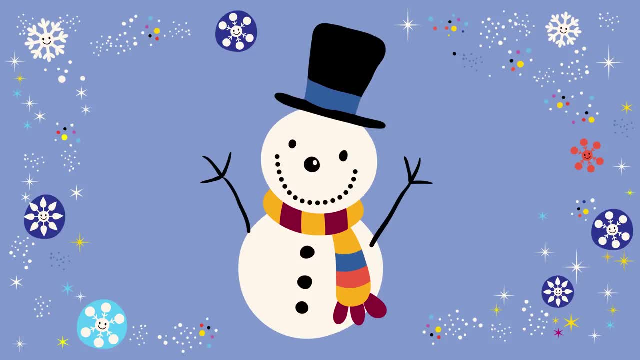 You follow the snowflakes As they flutter down from the sky and land on the ground. There's so much It's starting to make a carpet of soft, powdery snow. As you watch, the world outside begins to turn white. 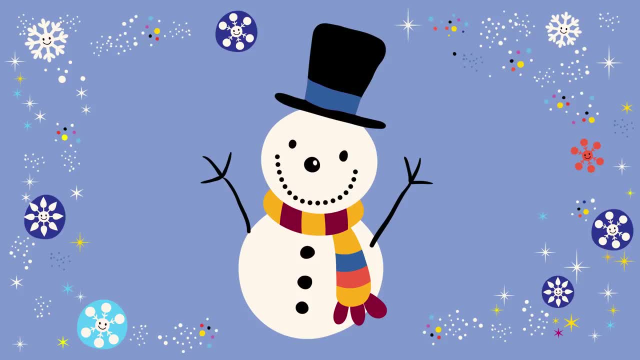 You have an idea? I'm going to build a snowman. Yes, You put on your coat, Your boots, your gloves, a scarf and a hat. Ready Out, you go into the garden. The air is chilly and fresh. 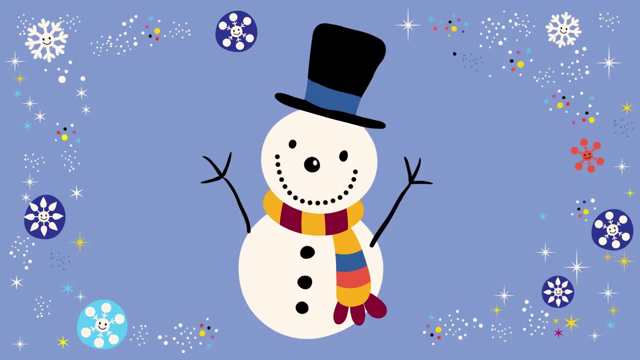 You run excitedly, enjoying the way the snow crunches under your boots. You stop and stand still for a moment. When it's snowing, it's so quiet. There's no sound of cars or birds. It's like everything is under a big blanket. 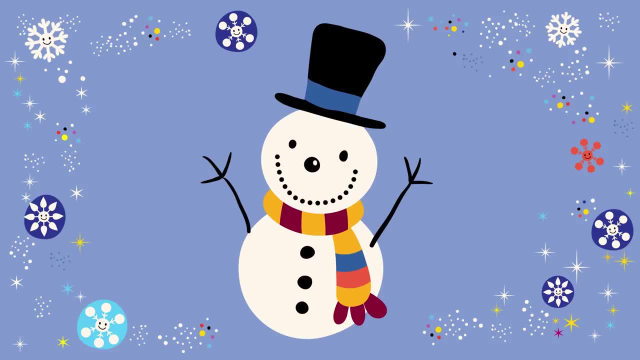 You lift your face to the sky With your eyes closed. you feel the snow gently pitter-pattering on your face. You open your mouth to catch snowflakes on your tongue. The snow turns to ice-cold water. It feels nice. 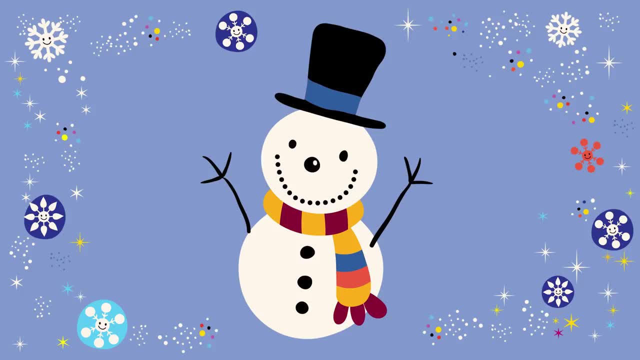 Refreshing Time to get started with your snowman. You get to work rolling giant snowballs to make the snowman's body and head. You give him sticks for arms and make his face, Adding two pieces of coal for his eyes, some little stones to be his smile. 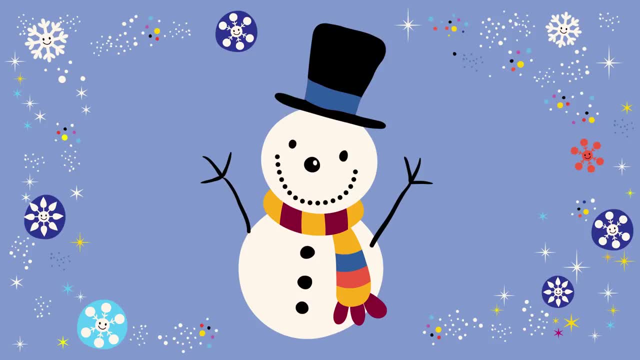 And finally his carrot nose. There you feel so pleased to have made him and stand back to admire him. What a proud snowman he is. You head inside to warm up and enjoy a hot chocolate. From the window you can see the snowman enjoying the garden. 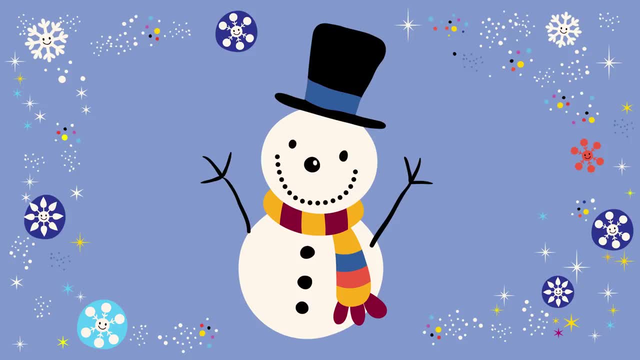 And for the next couple of days he stands tall and strong, Even though now the snow has stopped. On day three, you wake up to a bright, sunny morning. How lovely is the blue sky. You remember the snowman and run to the window to see. 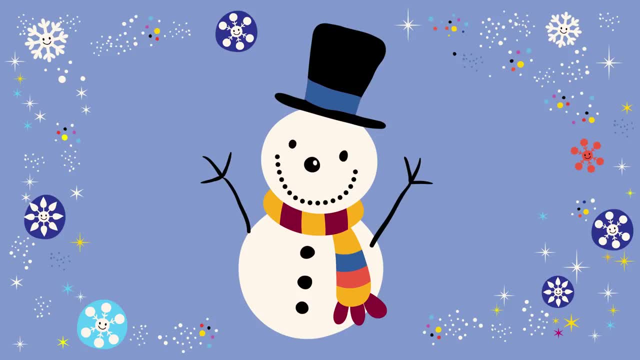 There he is. Only now. he seems to be smaller. He's melting. Once you're dressed, you go out to see him. He glistens in the sunlight, The frosty snow sparkling as it melts. For a moment you feel sad. 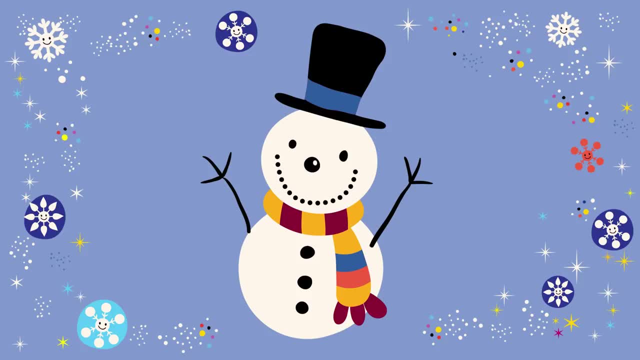 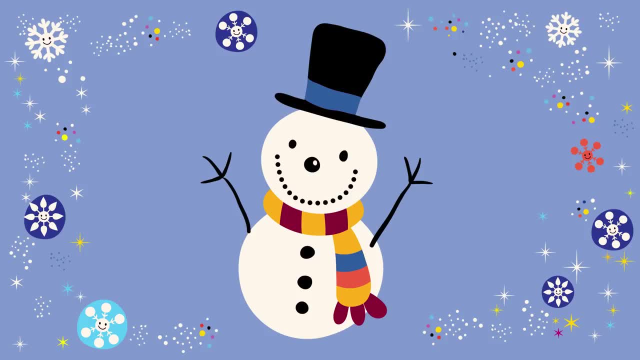 He's gone, You consider how to be. Do you get upset and feel sad about the snowman melting, Or do you let him go, Accepting that this is what happens, It's natural, And save yourself from feeling bad. Letting go may feel like a hard thing to do. 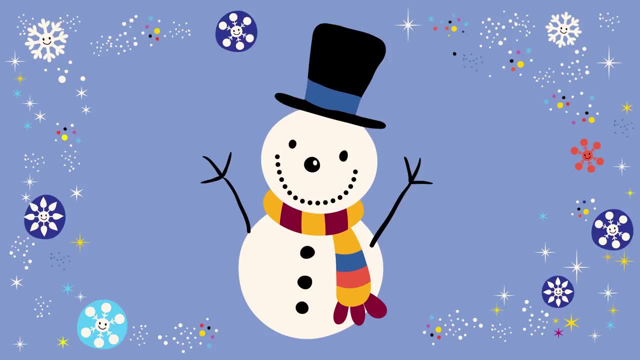 But in some ways it feels right. We are very good at getting things, But it takes extra strength and practice to let go of things. Much in our life is about letting go, Learning to be okay when we don't always get what we want. 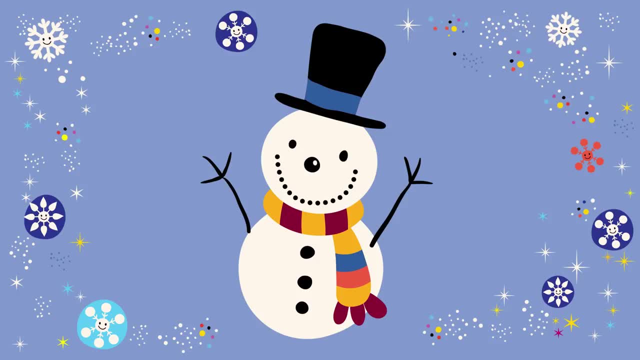 When we accept this, our life becomes easier, And we then appreciate something even more when we have it Just like the snowman: How much we loved him while he was here and how we will remember him sometimes, And that will make us smile. 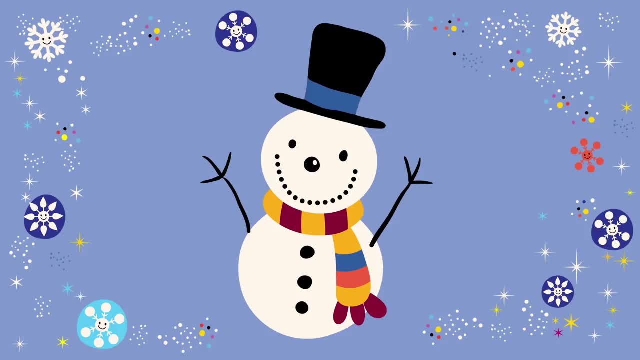 Slowly now begin to come back to the present moment. Take a deeper breath and wiggle your arms. Think about the things that you do for him. Say I love you, I love you so much, I love you so much. 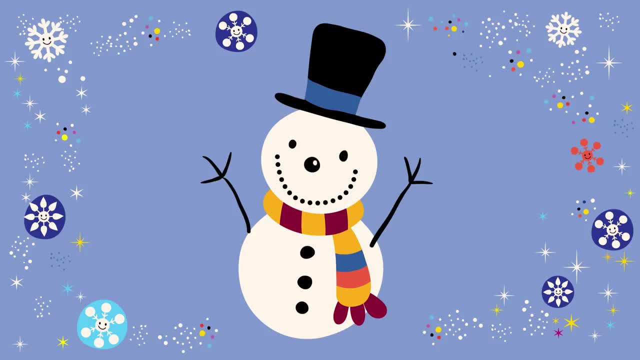 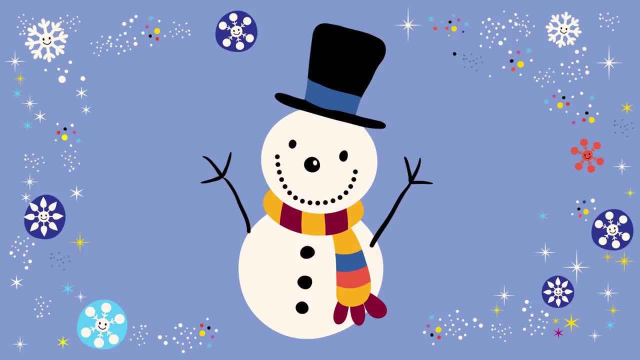 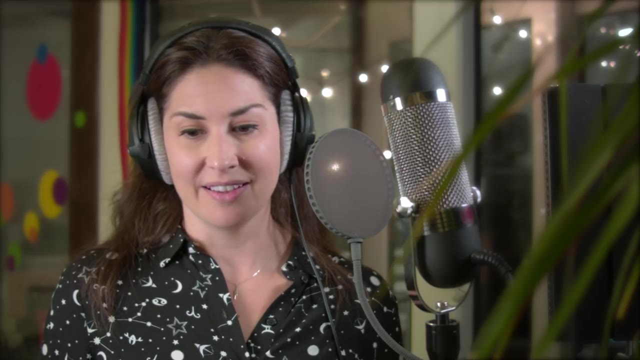 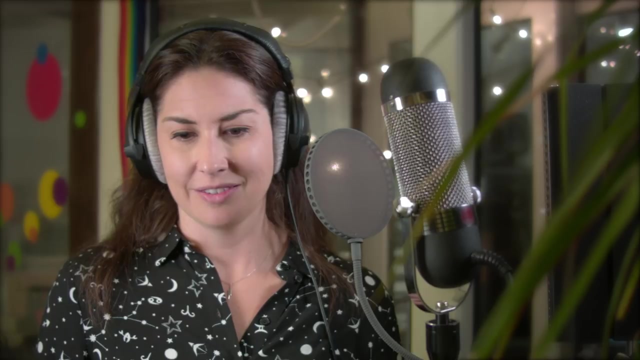 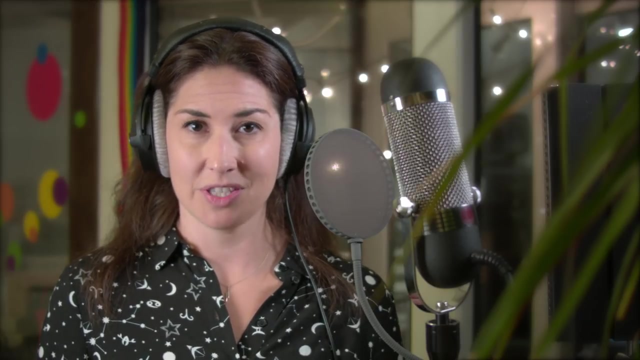 wiggle your fingers and toes, Enjoy a stretch and slowly, gently open your eyes, letting the world back in again Before moving anywhere. just sit for a moment here and notice how you feel, Your body and mind, thanking you for this time, this peaceful time, just to.